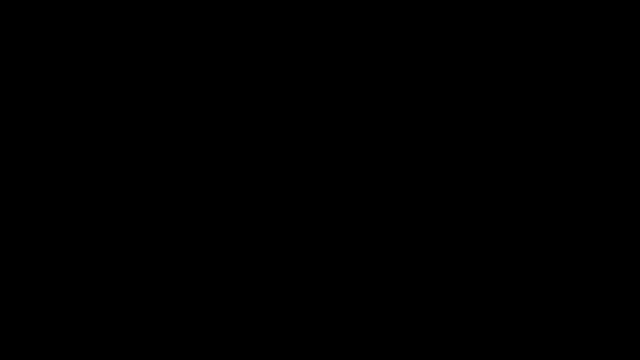 In this video we're going to talk about the second part of the Fundamental Theorem of Calculus. Now, some books may call it the first part, but you can go with whatever your textbook says. So the basic idea is that you have a function f. 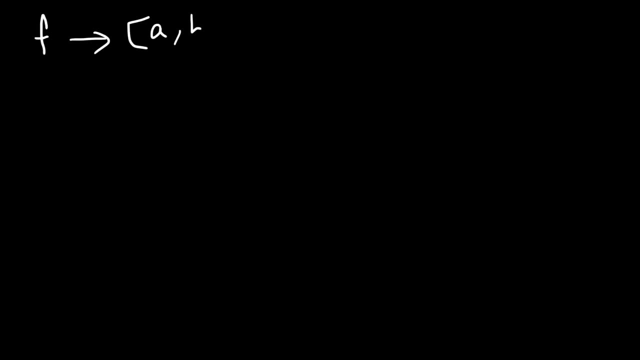 and it's continuous on the closed interval a, b and capital F represents the antiderivative of lowercase f. So in that case then, according to the Fundamental Theorem of Calculus, the definite integral of f, that's lowercase f, on the interval a to b, that's equal to f evaluated from a. 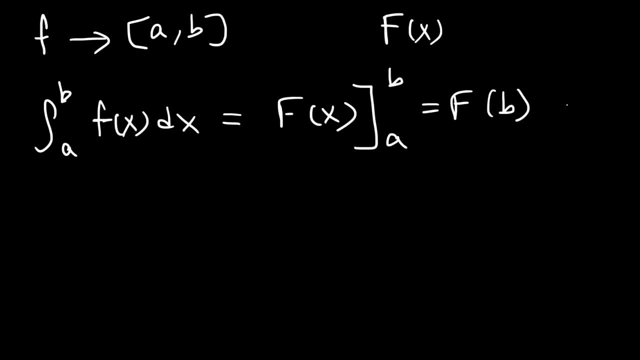 to b, which is f minus f. So this theorem describes the process by which we can evaluate a definite integral. So let's go over some examples, Go ahead and evaluate this particular integral. Feel free to pause the video if you want to try it. So the antiderivative of 3x. 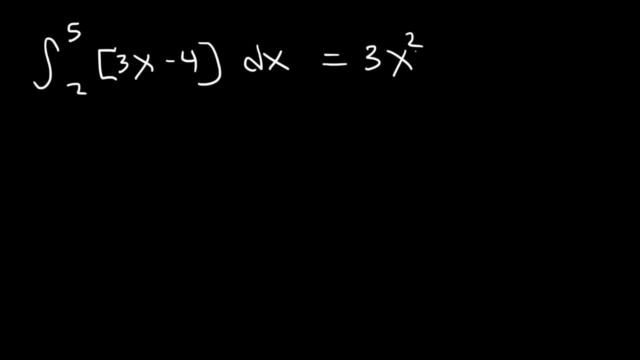 using a power rule is going to be 3x to the second power divided by 2 and the antiderivative of 4 is 4x. So let's evaluate it from 2 to 5.. So f of 5 is going to be 3 times 5 squared over 2 minus 4 times 5 minus f of 2.. So if we 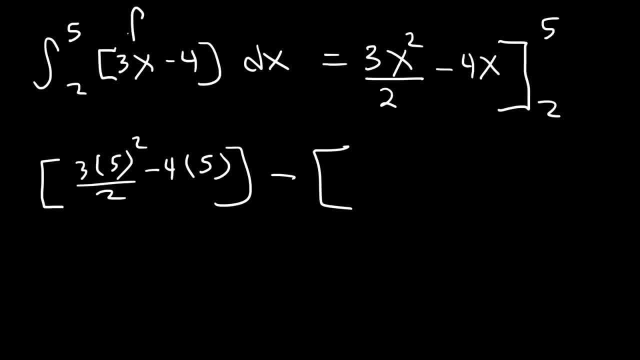 plug in 2 into f of x. Now keep in mind this is lowercase f of x and this represents the capital F of x, the antiderivative of f. So this is f of 5 minus f of 2.. So that's going to be 3 times 2 squared over 2 minus 4 times 2.. Now 5 squared is: 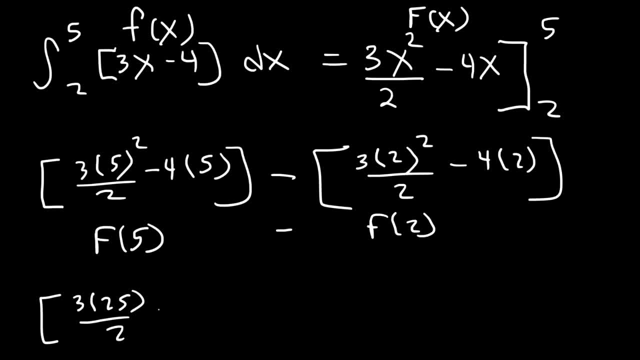 25.. 4 times 5 is 20.. 2 squared is 4, divided by 2, that's 2, and 3 times 2 is 6.. 4 times 2 is 8.. Now, 3 times 25 is 75.. 6 minus 2 is negative, 2 times this negative. 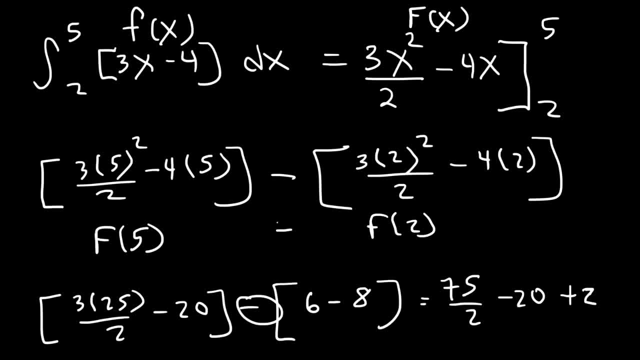 sign. So that's positive 2.. Negative 20 plus 2 is negative 18.. Now we need to get common denominators. So this is going to be 75 over 2 minus 36 over 2. And 75 minus 36,, that's going to be 39. And 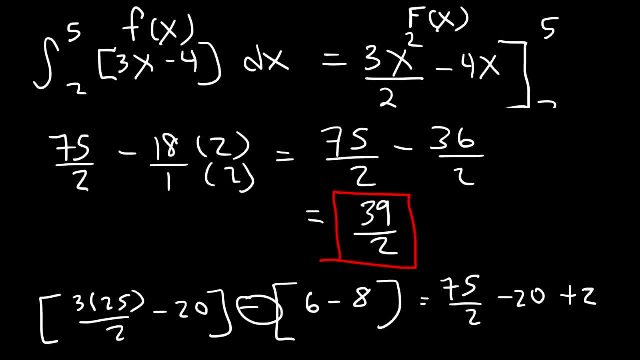 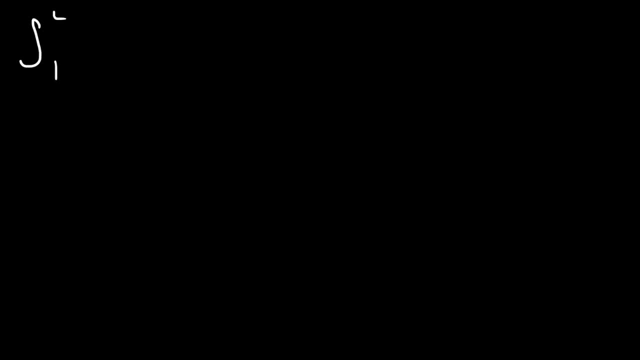 And that's the final answer: 39 divided by 2.. Let's work on some more examples. So use the second part of the fundamental theorem of calculus to evaluate the definite integral. Now, before we could find the antiderivative, we should FOIL this expression. 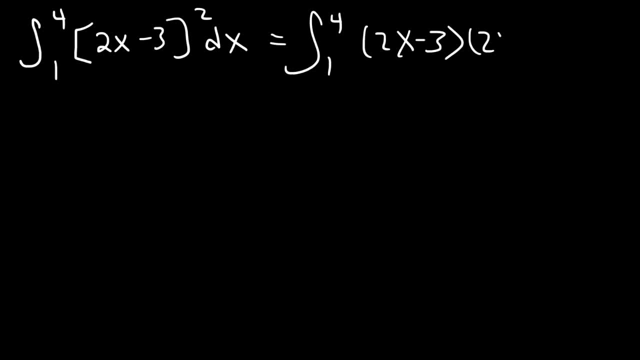 So what we have is 2x minus 3 multiplied by another 2x minus 3.. So first we have 2x times 2x and that's going to give us 4x squared. Then it's 2x times negative 3, so that's negative 6x, and negative 3 times 2x is negative 6x. 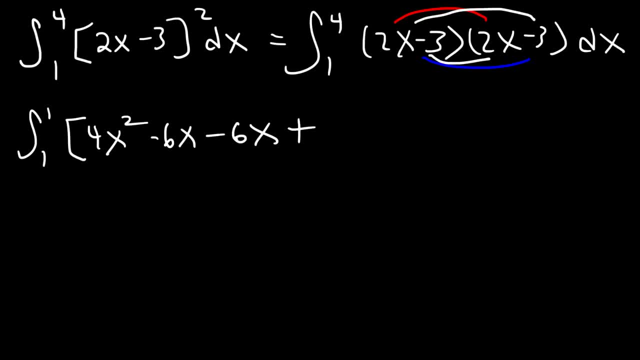 and then negative 3 times negative 3, that is positive 9.. So now what we need to do is combine like terms, and this is supposed to be a 4. Negative 6 minus 6 is negative 12. So this is what we now have. 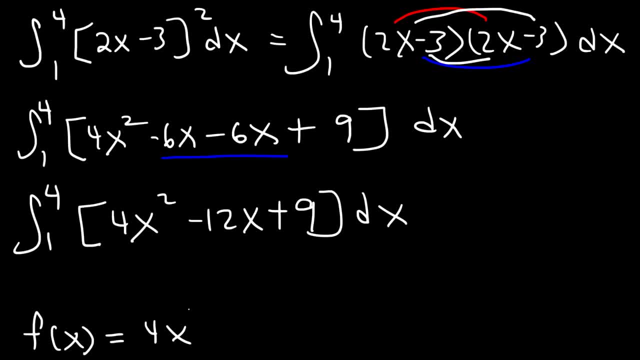 Now lower case f is 4x squared minus 12x plus 9.. Now we need to find the antiderivative capital F of x. So we're going to find the antiderivative capital F of x. So we're going to find the antiderivative capital F of x. 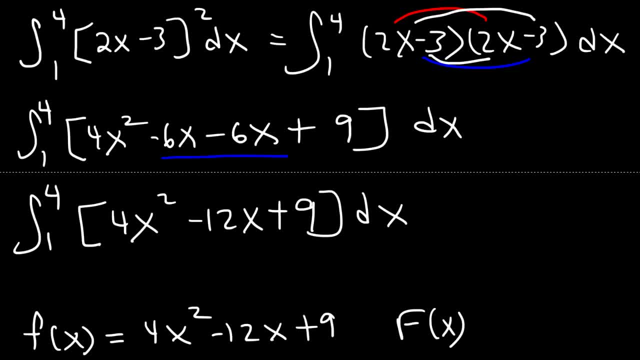 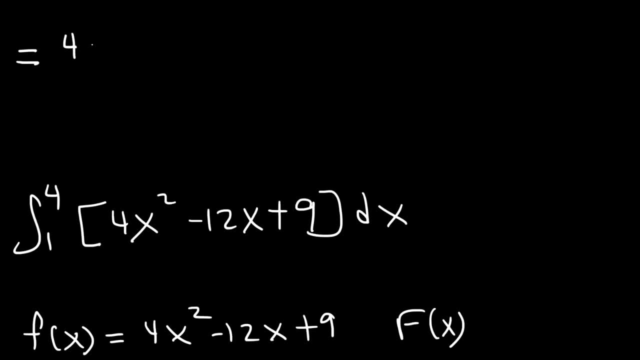 So we're going to find the antiderivative capital F of x. Now let's start at the top. So the antiderivative of x squared is going to be x cubed over 3, and for x it's x squared over 2, and the antiderivative of a constant is going to be the constant times, the variable. 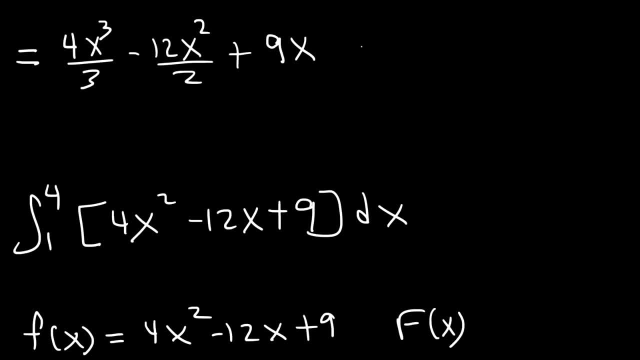 of integration, which is x. So this is capital F of x, And we're going to evaluate it from 1 to 4.. So what we have now is F of x 1 to 4. And that's equal to F of 4 minus F of 1.. 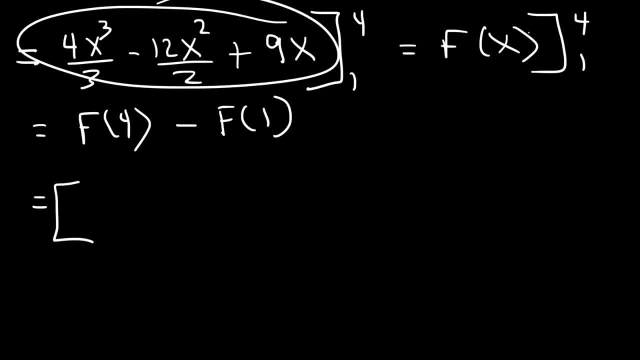 So let's start with F of 4.. Let's plug in 4 into that expression, So it's going to be 4.. So it's going to be 4 times 4 raised to the third power divided by 3.. And 12 divided by 2 is 6.. 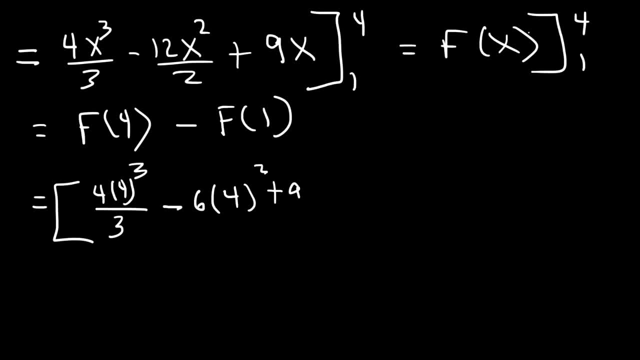 So it's going to be 6 times 4 squared plus 9 times 4. And then minus F of 1.. So 1 to the third is 1 times 4 over 3. And 1 squared times 6 is just 6.. 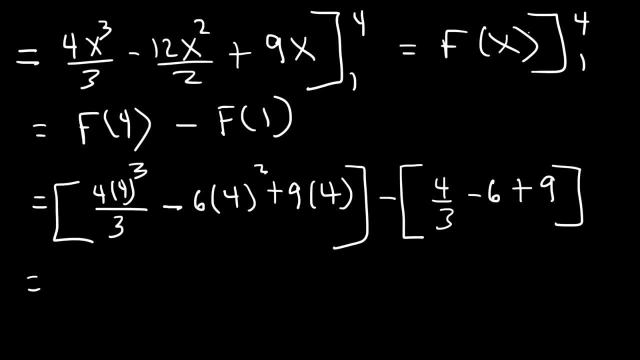 And then plus 9 times 1 or 9. And then minus F of 1.. So 1 to the third is 1 times 4 over 3.. Now 4 to the third power, That's 64. And if we multiply that by 4, we're going to have 256 divided by 3.. 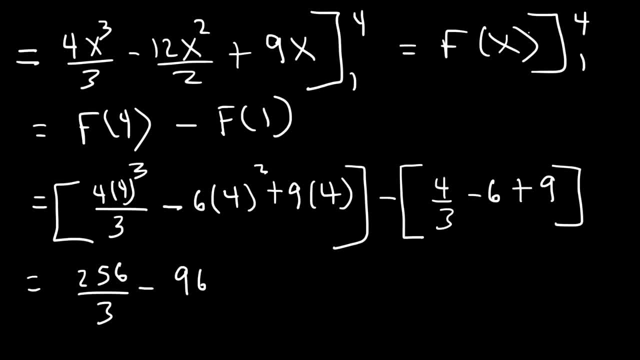 4 squared is 16.. 16 times 6 is 96.. And 9 times 4 is 36.. And then we have minus 4 thirds, And if we distribute the negative sign, plus 6, minus 9. That's negative 3.. 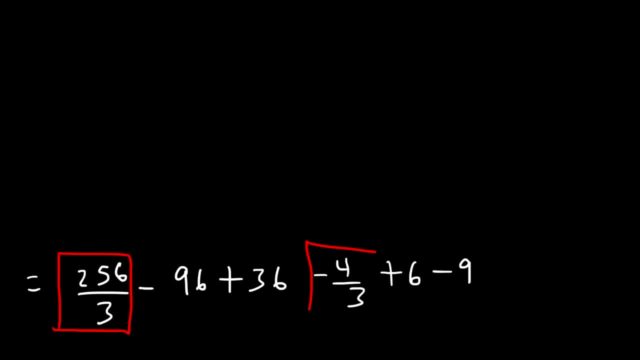 So the first thing we could do is combine these two fractions, because they share the same denominator: 256 minus 4 is 252.. Negative: 96 plus 36.. That's negative 60.. And 6 minus 9.. That's negative 3.. 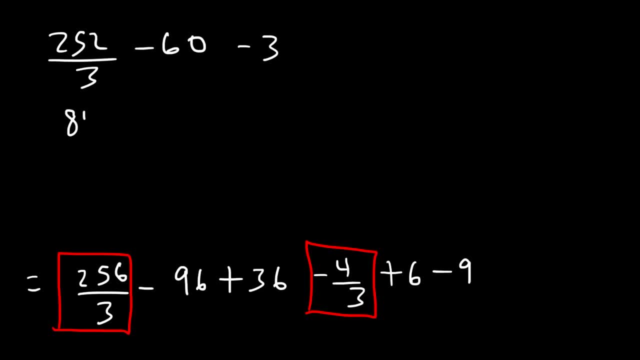 Now, 252 divided by 3 is 84.. That's negative 3.. Now 252 divided by 3 is 84.. That's negative 3.. And 60 minus well negative. 60 minus 3 is negative 63.. 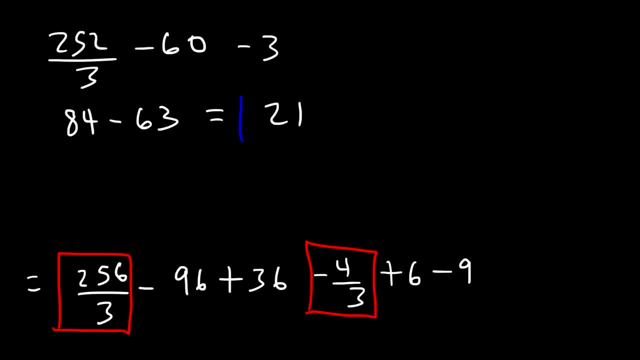 So 84 minus 63 is 21.. And that is the final answer. Let's work on this example. Find a definite integral from 1 to 4 of the square root of 5 over x. So what do you think we should do in this problem? 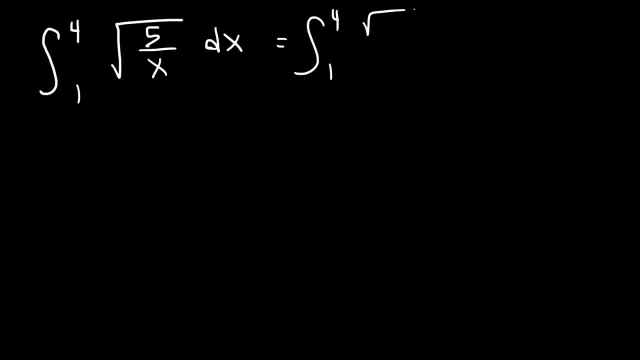 Well, first We can rewrite the expression like this: It's equivalent to the square root of 5 divided by the square root of x, And the square root of 5 is a constant Which we can move that to the front. So this is what we now have. 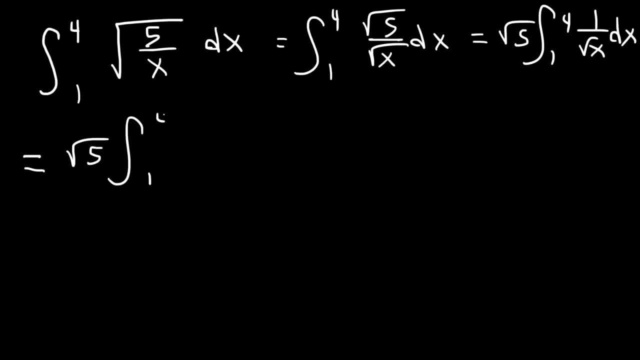 We can rewrite the square root of x as x raised to the 1 half And we're not done rewriting, So now Next variable: we'll move it to the top, So we could use the power rule. So this is x raised to the negative 1 half. 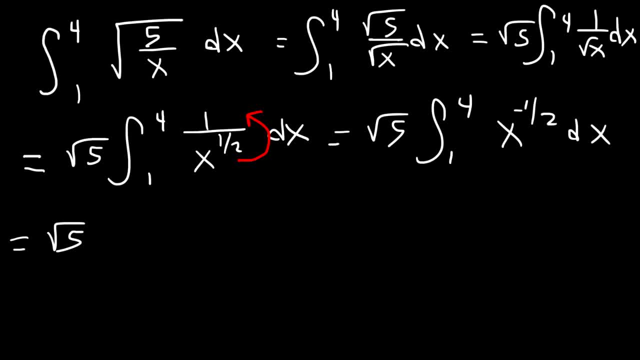 And now we can use the power rule. So negative: 1 half plus 1 is 1 half. And then we need to divide that by a half, Which, if you multiply the top and bottom by 2 over 2.. 1 half times 2 is 1.. 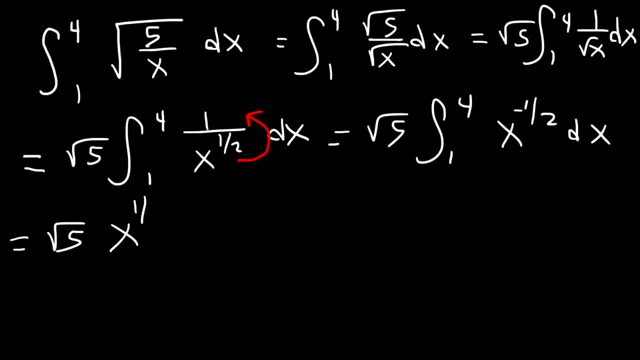 So we can just put the 2 on top And that's it. Now we're going to run a little bit of running around And we're going to evaluate this from 1 to 4.. So what we now have is 2 square root 5.. 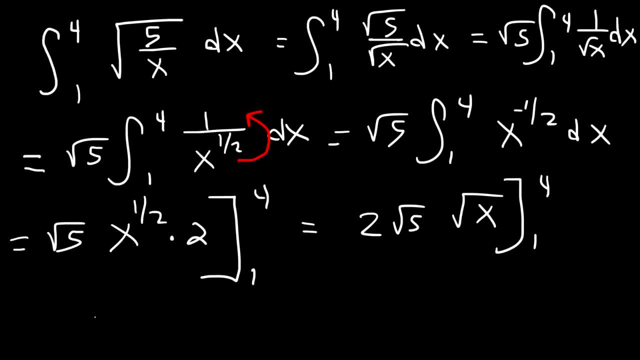 Times the square root of x from 1 to 4.. So let's plug in 4 first And then we can plug in 1.. So the square root of 4 is 2. And the square root of 1.. Well, that's 1.. 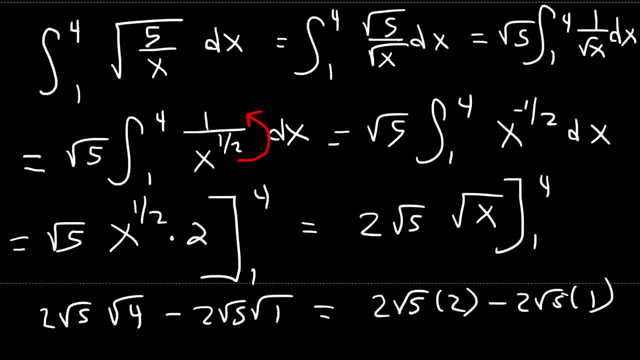 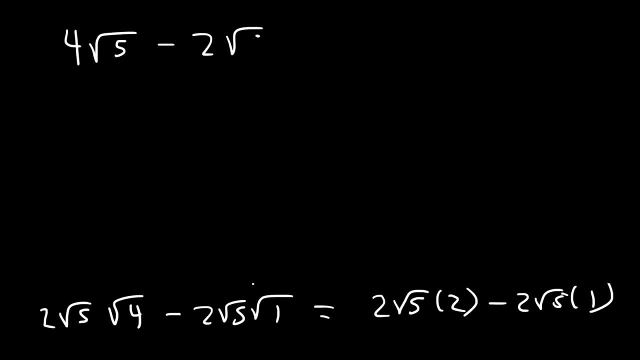 2 times 2 is 4, so we have 4 square root 5, and 2 times 1 is 2, and then we could subtract the coefficients, so 4 minus 2 is 2, so the final answer is 2 square root 5, and that's it. let's work on one final problem. use the fundamental.